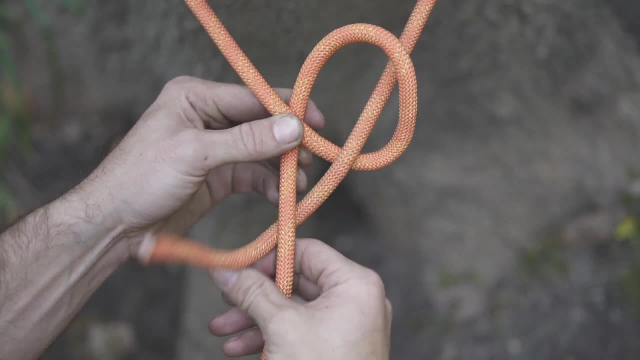 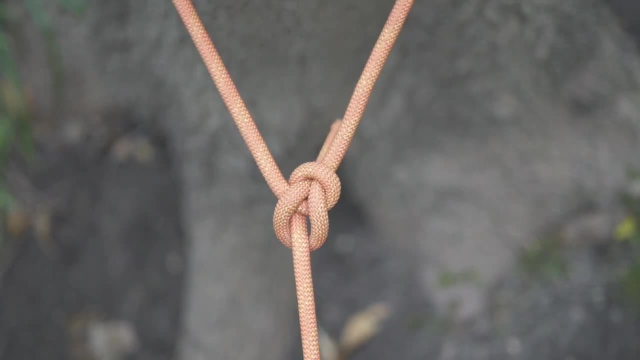 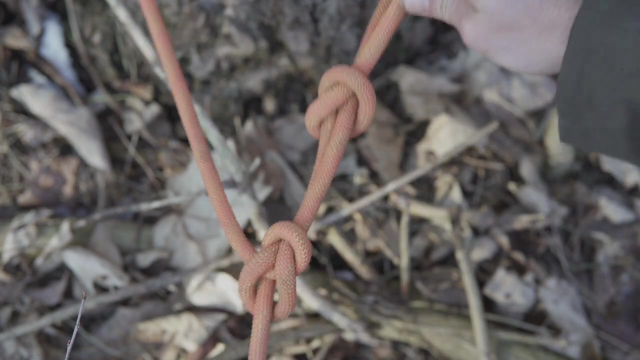 And to tighten, you just pull all the ends and you have your bowline. The knot should look like this: with that definitive U-shaped wrap there, That tag end will be inside the loop and some people will tie a safety knot with it for added security. Now, if you accidentally wrap around the 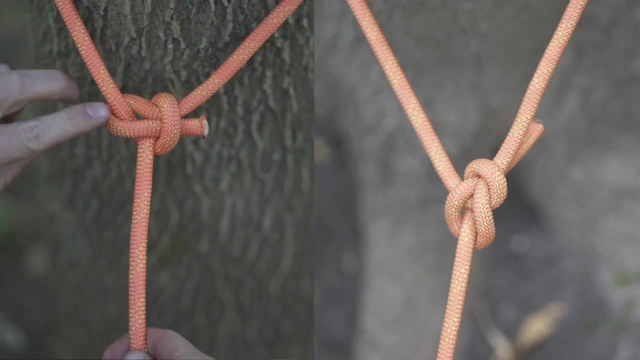 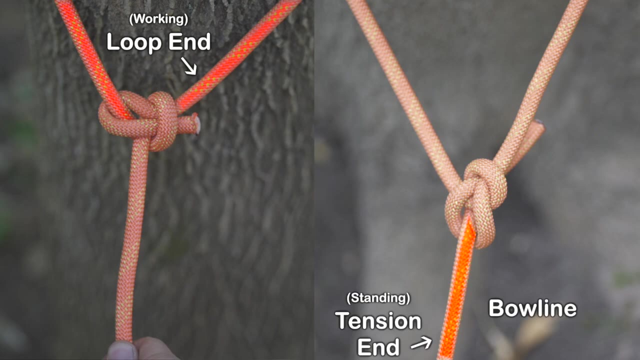 wrong line. it could turn out like this: The knot itself looks the same, but it's wrapped around the loop end and not the tension end, where it's supposed to be. Never fear, though: if you've accidentally tied this, then you've accidentally tied the wrong line, and you've accidentally 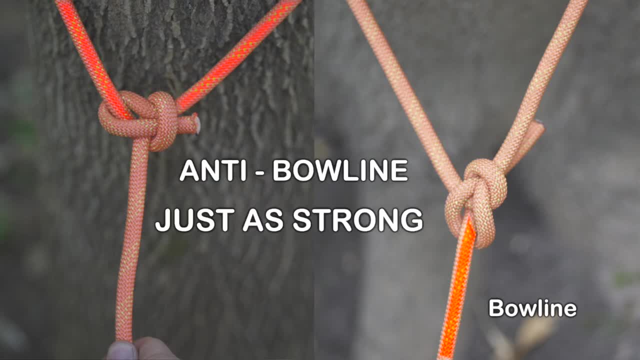 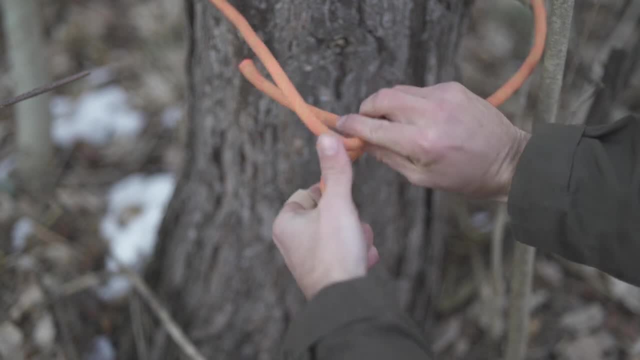 tied the anti-bowline knot, which is just as strong and arguably even more secure than the original bowline. To tie it a little bit faster, you could keep the free end in your hand as you go through that wrist motion of the car turning off and it's already in position to be wrapped. 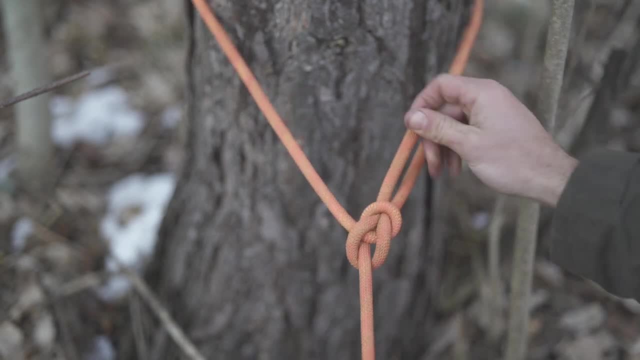 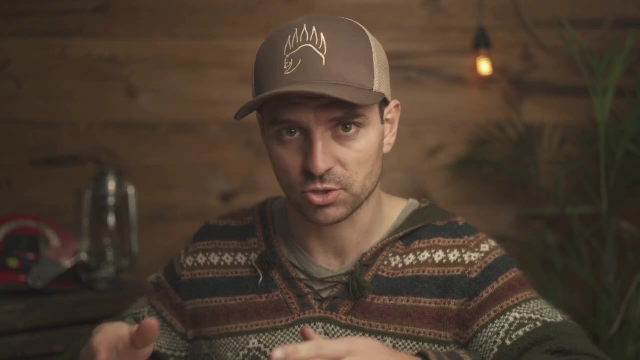 around and back underneath, just like normal. While it's great to learn a knot in a single direction, it's important to remember that when that knot flips, or you're tying it away from you versus towards you, that technique is going to change a little bit, And that's one thing. 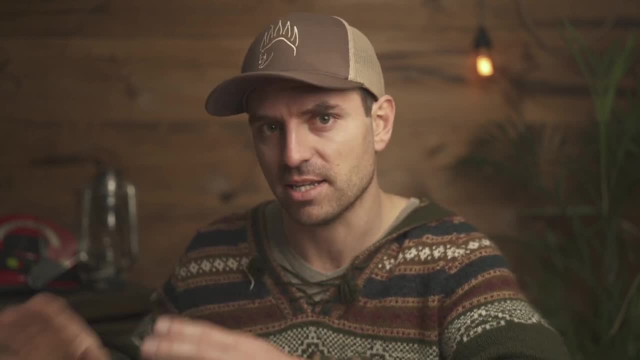 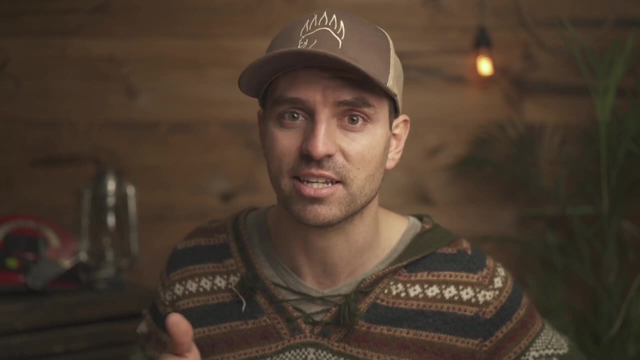 I personally struggled with tying a knot, facing myself or facing the other way. How exactly do you remember how to do each knot? Well, what helped me was using association and various techniques that I could stick to just like this, For instance, tying around a backpack or a tent. 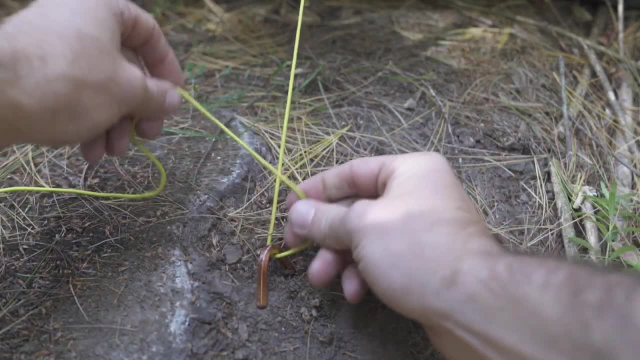 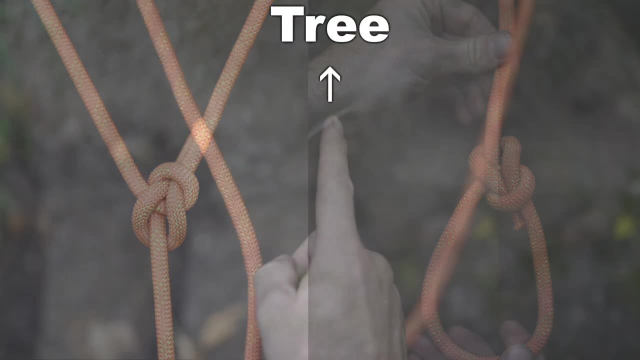 peg where the object's closer to us and then that tension line is farther away from us And so, depending on where the object is, that knot itself is going to be turned around and facing the opposite way. So initially there was that tree in front of us, so we had to turn the car keys off. 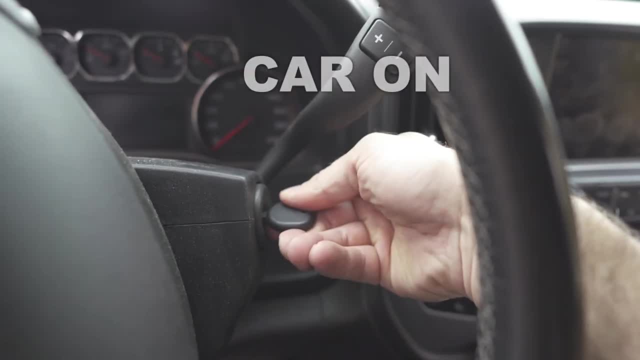 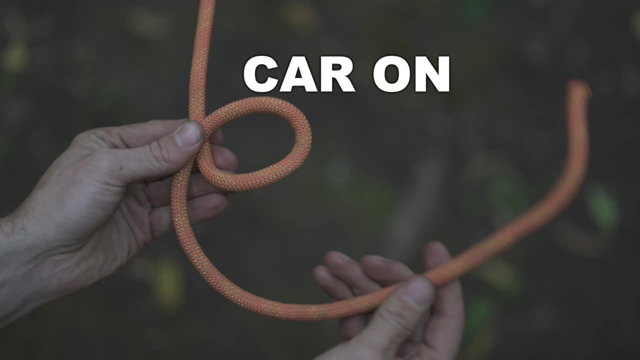 But now we have open space in front of us so we can turn the car keys on And with that wrist motion we're going to use it on our standing line to create the loop there. Now, the rest of the steps are pretty much the same, And there's even an old saying to help you remember this part. It 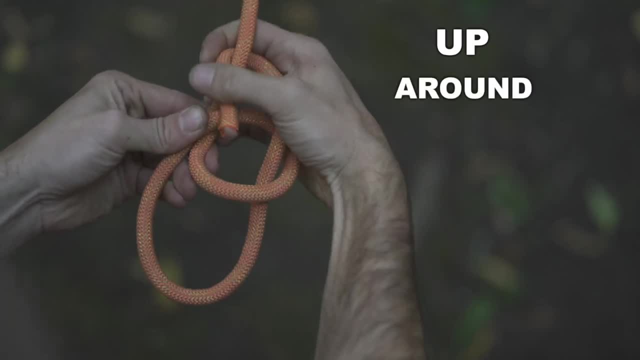 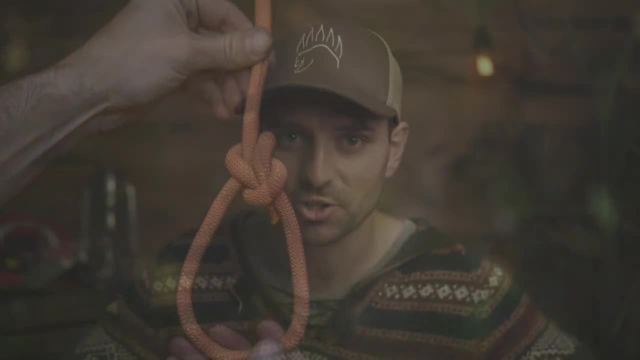 goes like this: The rabbit comes up through the hole, runs around the backside of the tree and back down into its hole. Now, as I mentioned earlier, here are a few more practical ways in which to use the bowline. One of them is simply to connect two lengths of rope.